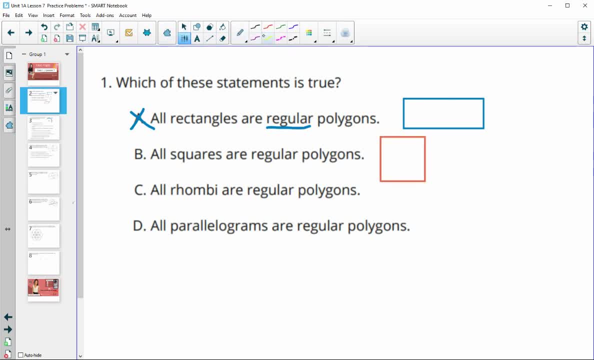 All squares are regular polygons. So again we've got that word regular, equilateral and equiangular. A square certainly is equilateral And it is also equiangular, So this is going to be a true statement. Let's just look at the others just to make sure. So all rhombi meaning the plural of rhombus. 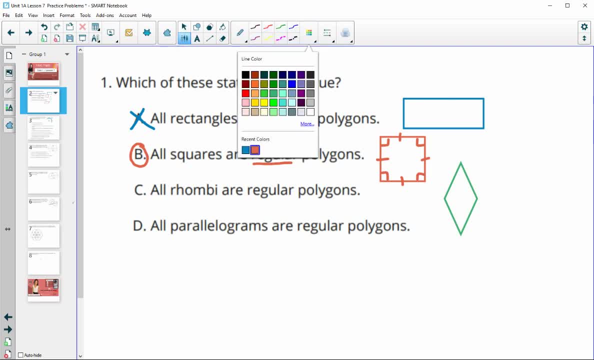 So all rhombi are regular polygons, And in this case we've got equilateral but not equiangular, So that's definitely false. And then parallelograms are regular polygons, And then we've got equilateral but not equilateral, So that's definitely false. 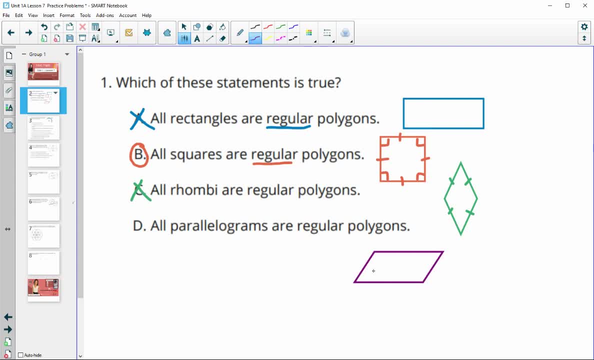 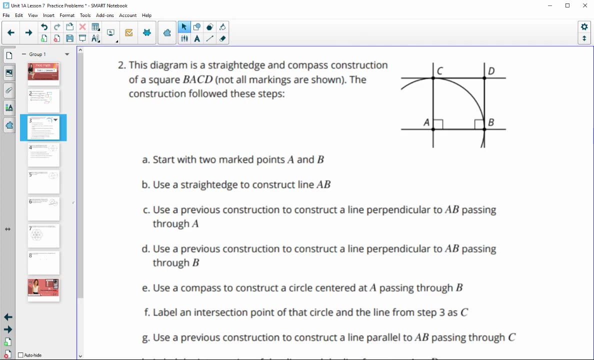 That is going to be false as well. Parallelograms do not need to be equiangular or equilateral. Could be, but don't have to be. So all squares are regular polygons, would be the true statement. there, All right. Number two gives us a straight edge and compass. construction of square. BACD Doesn't. 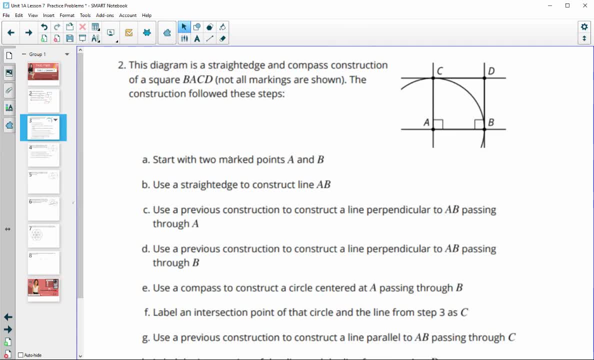 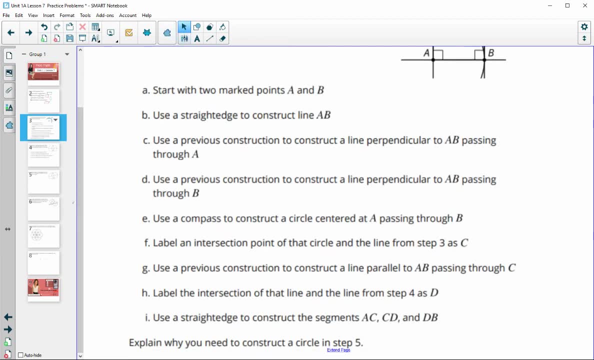 have all of the construction markings showing, And then it tells us that it follows these steps here. And then it tells us that it follows these steps here. And then it tells us that it follows. And then they want us to explain why you need to construct the circle in step five. So let's take a 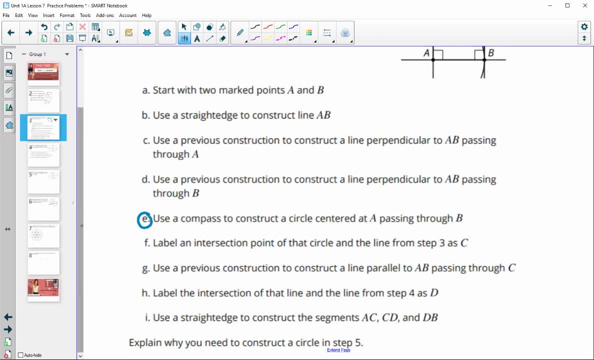 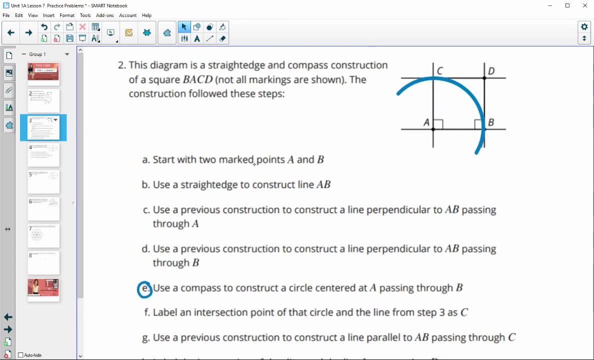 look at step five, which would be E. So why do we need step five? Why do we need to construct this circle here? So first of all let's look at these. first construction. So it says start with two marked points. So we're starting just with A and B. So if we kind of drew this off to the side, 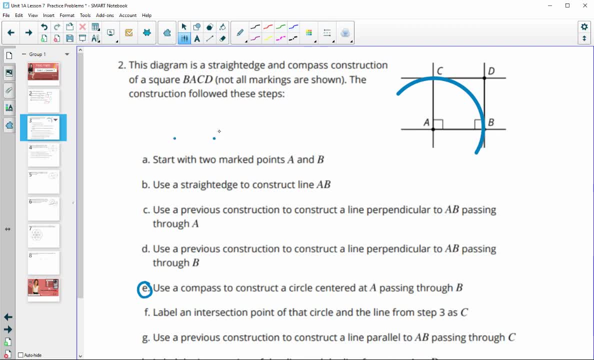 we would be starting with just A and B And then we're going to use a straight edge to construct line AB. So then we connected those two points. Then we're going to use this previous construction to construct a line perpendicular to AB through A. So remember that. 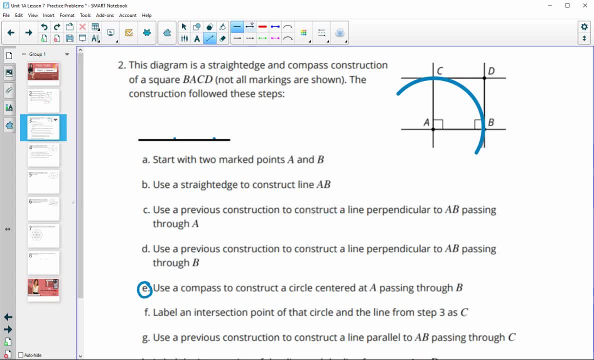 would be- and I'm not going to use, I'm just going to draw it with a circle tool- but you would use a compass to draw a circle around here And then you would use a compass to go through the intersection points And then that would get you your perpendicular line through A. 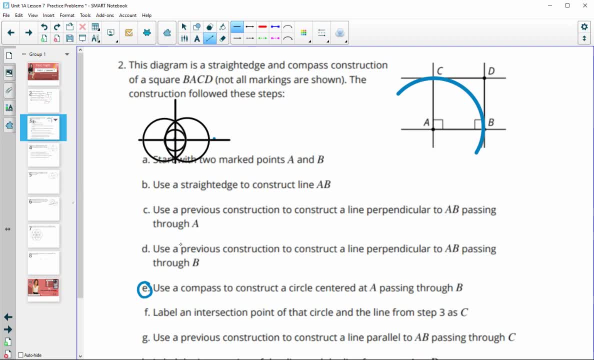 Okay. So now we've got that perpendicular line through A, Then it says to do this again to get the line through B. So I'm just going to draw it there. And so now it's asking: why then- okay, after we've gotten all of this done- why do we need to take and use the compass to draw a circle? 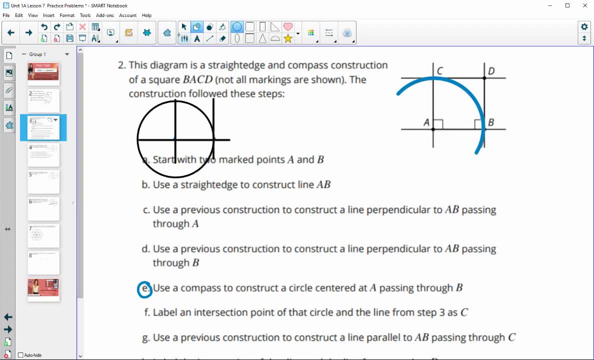 here. Why do we draw this circle? And the reason being is that then we're setting this radius, So now we're going to use a compass to draw a circle here. So now we're setting this radius, So now we've. And the reason being is that then we're setting this radius, So now we're setting this radius, So now we're. 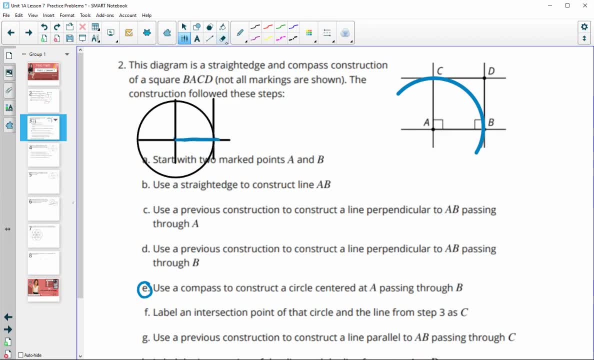 we've made this the radius right, which is the length of AB, And so now any radius in this circle is going to be that same length. So now we know that this segment here is going to be the same length as AB, since they're both radii. So that's the point of that circle. 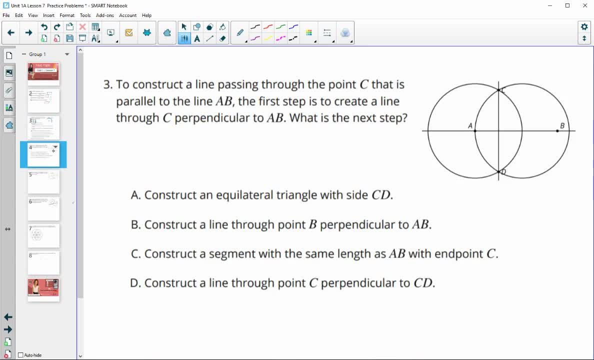 Number three, to construct a line passing through point C that is parallel to AB. the first step is to create a line perpendicular to C or sorry, perpendicular to AB through C. So to create this line right here, let me get a different color. So our first step was to get 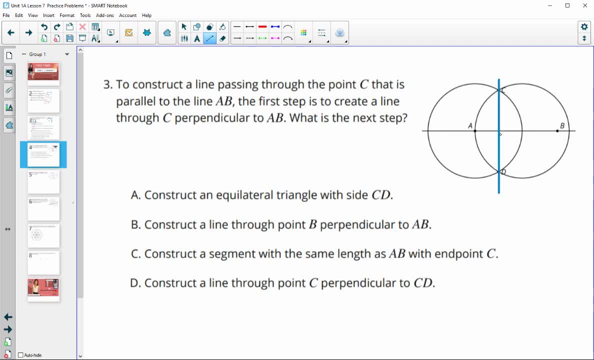 this perpendicular line that goes is perpendicular to AB through C. What's the next step? So, if we're trying to get this parallel line- so let me just draw the parallel line here- So we're trying to do this, So what would our next step be? So we're going to do this. So we're going to do this. 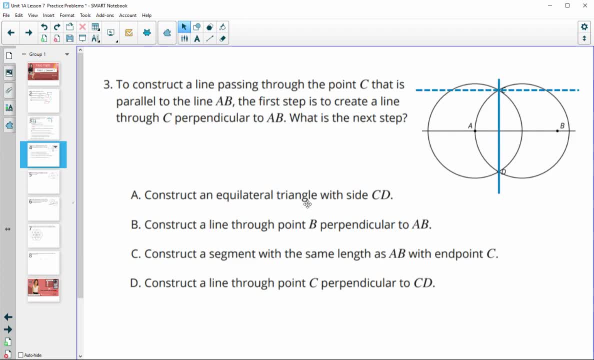 Next step B: construct an equilateral triangle. So a triangle isn't going to do us any good. Construct a line through B that's perpendicular to AB, So we could do this, but that doesn't seem to help us get this parallel line. Construct a segment with the same. 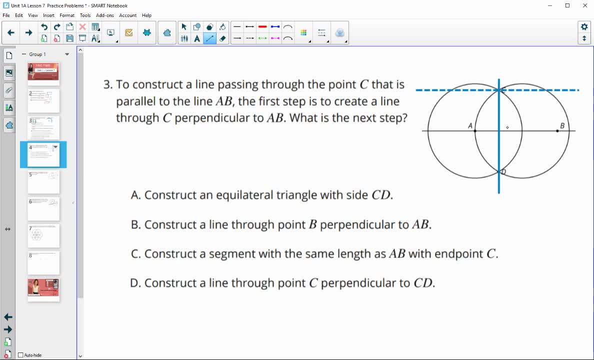 length as AB, with end point C. So construct just any segment. Well, it could be like this: Okay, If it's going to be the same length as AB, you just set your compass open it. You could get any segment around here. That doesn't guarantee that it is going to be parallel to AB. 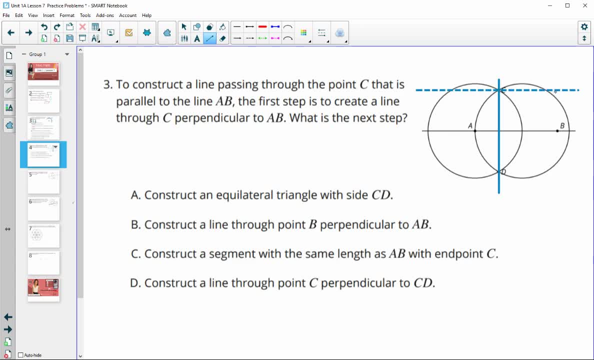 Construct a line through C that is perpendicular to CD. So that would work, Because if we do this line, it's going to be perpendicular here, Okay, So perpendicular to the perpendicular line that's going to force these two to be parallel. So it would be D. 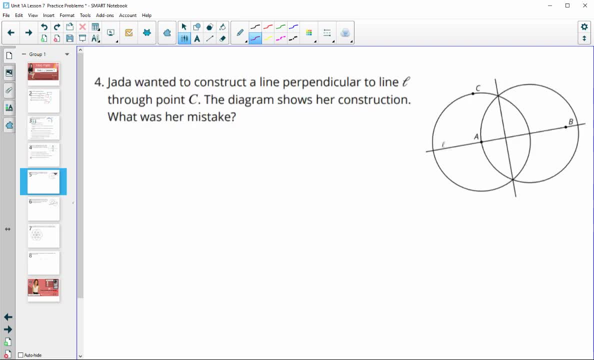 Number four: Jada wanted to construct a line perpendicular to line L through point C. The diagram shows her construction. What is her mistake? So it looks like Jada, you know, drew her initial circle here, So let me get this in a color. So she went, she drew, it looks like she. 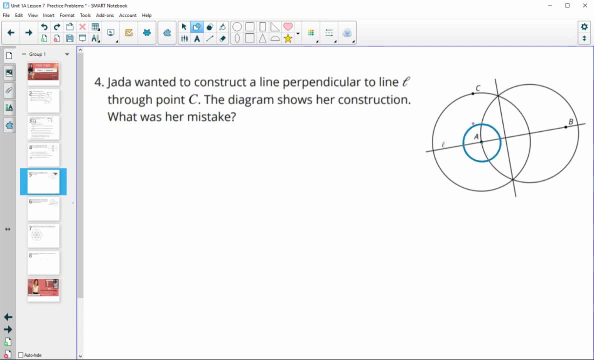 drew a circle from C, right Or not from C, but centered through A. So she kind of drew this And then she just drew another circle somewhere. I'm not sure, But what she needed to do, okay, was get a circle- whoopsies, get two points or a circle drawn from C. So let me 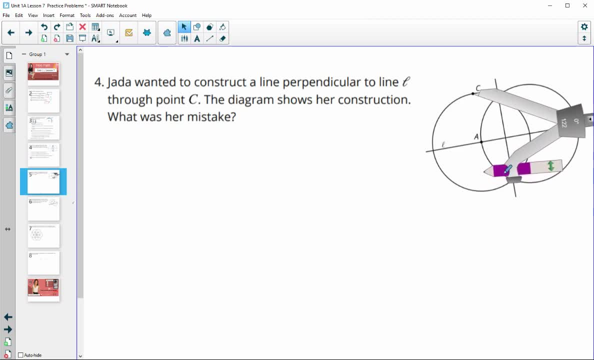 get this here so that she could set kind of two marks here- And let me make it smaller so it actually hits- So she could find two points that were in the middle of the circle And then she could draw a circle around here, a circle around this one, then connect those two And that's. 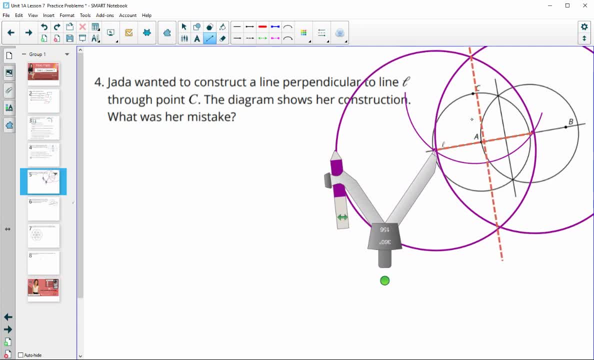 going to force C to be on that perpendicular bisector, So we can type that out. So, Jada, let's see, let's get this a little bit smaller. So Jada needed to find two points the same distance from C that are on line L. 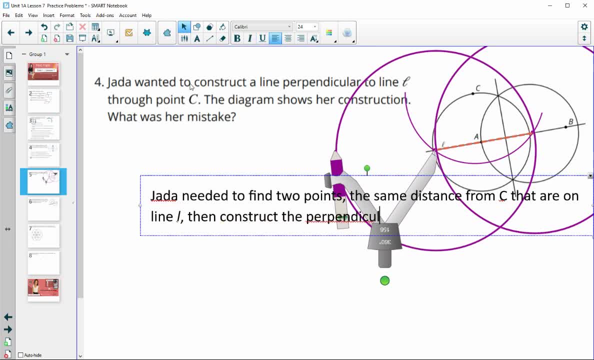 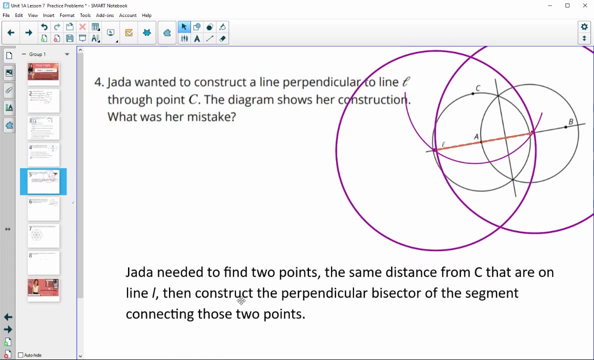 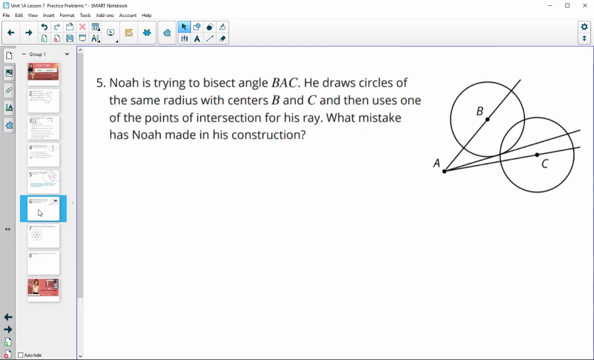 And construct the perpendicular bisector, So the perpendicular bisector of the segment connecting those two points. That would force C to be on that line. Okay, Number five: Noah is trying to bisect angle BAC. He draws circles of the same radius with 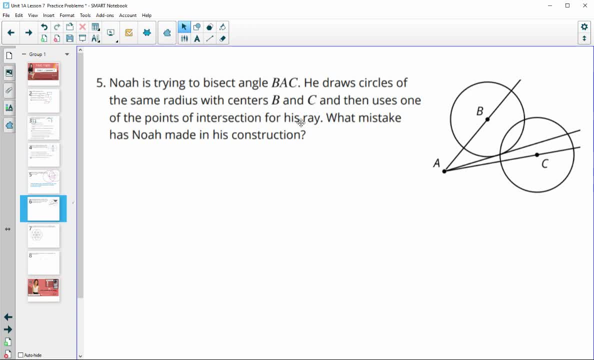 something pointing. the same way, He's drawing a circle with a respecto angle And then Jada centers at B and C, then uses one of the points of intersection for his ray. What is his mistake? So it's good, He wants to have these kind of two circles going around two points. The problem is: 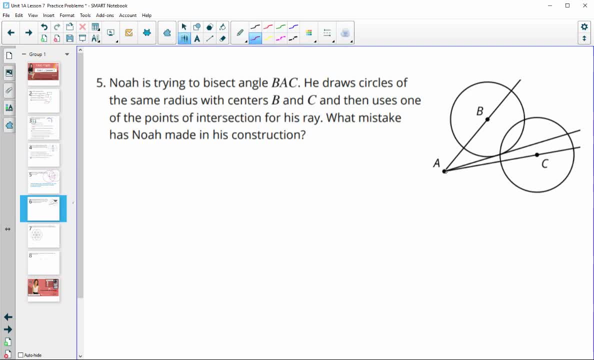 is that these two points need to be the same distance from A, So he can't just use any points, B and C. The two points need to be the same distance from A. So he would want to first, you know, draw a circle. If he wants to use B, that's fine, Then he needs to draw a circle. 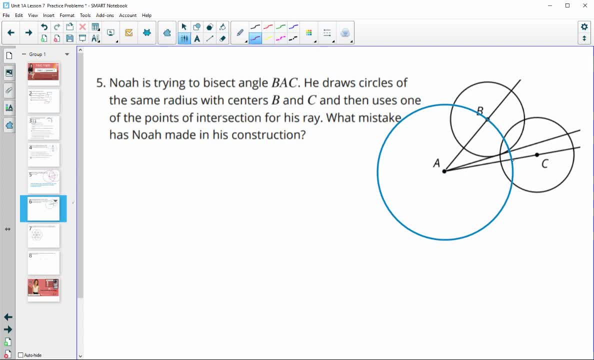 that goes through B, And then he'd need to use this point instead of C to draw his next. his circle congruent to this one, So if he then drew that circle around this point, then he could connect them. Obviously that's a bad circle, but 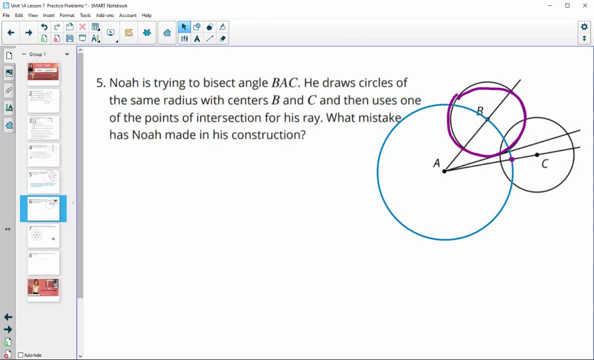 draw a circle around this new intersection point. So let's type that out. So Noah needed to use two points that are the same distance from A- one on each side or each ray of the angle- Then construct congruent circles around each of those two points. 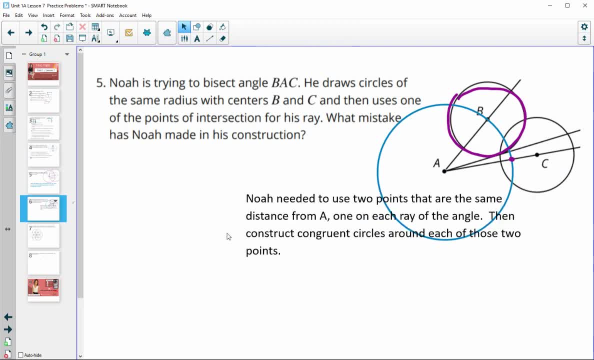 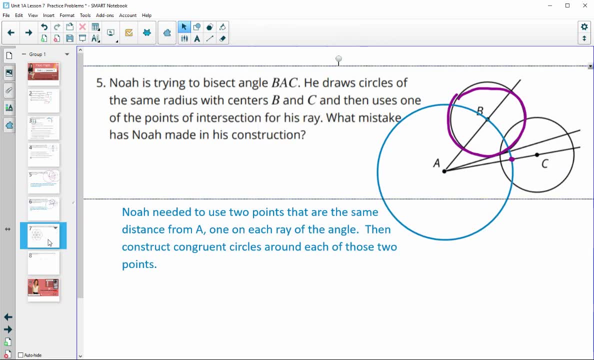 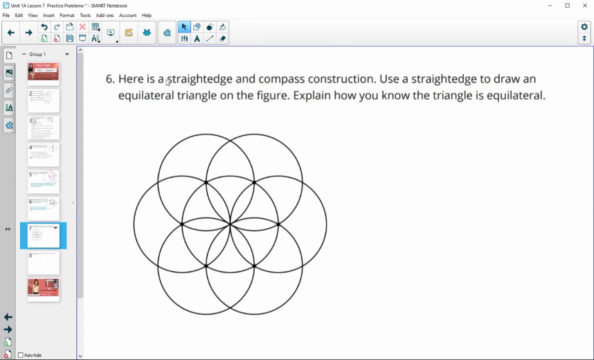 We've got to make sure that the points are the same distance from A before you start doing the circles around them. Number six: this is a straight edge and compass construction. Use a straight edge to draw an equilateral triangle on the figure. How do you know it's equilateral. Okay, so you. 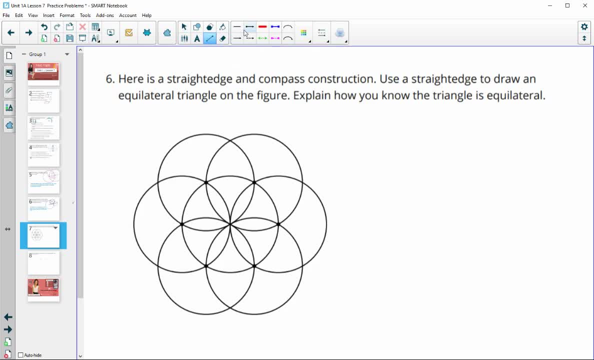 can do your equilateral triangle wherever you want, as long as you can explain it. So let me see what color we got here. So I'm just going to use radius to radius and actually let me make this a solid line. So here's the center of this circle. 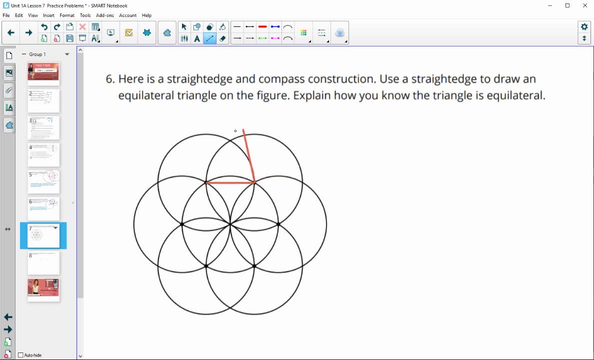 So I'm just going to connect it here to the edge. Now I've got the center of this circle, So I'm going to connect that to its edge and then I'm going to connect those. So these are all radii of the little circles, And so then that orange triangle is going to be equilateral. So that's. 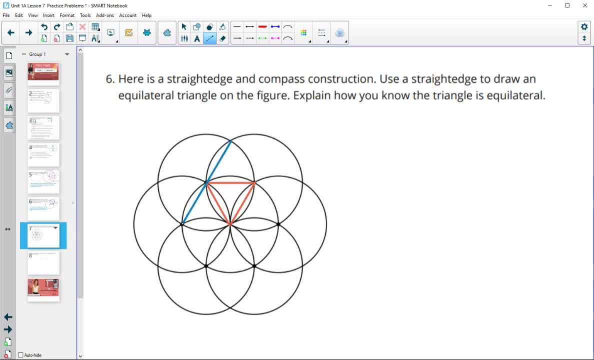 a Hebdry's jeito, I toss on in circles on my iris. So, depending on where we're going with this, it may sound old fashioned when you're doing this, but this is probably going to be the. instead of having the facelifted 케 regular after we're done here, you could do. 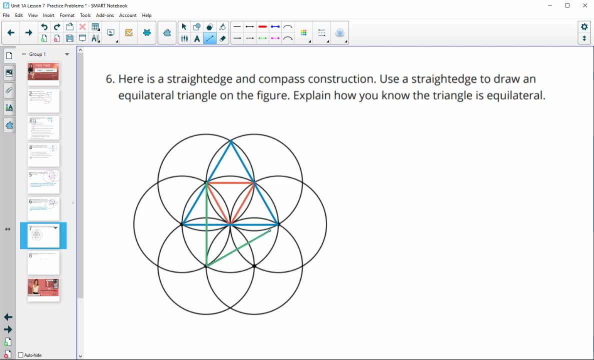 another. Let's see It's going to be a square one, so hopefully that's not because of theύ. To me this is going to be an equilateral triangle, because instead of is going to be the two pieces of paper. 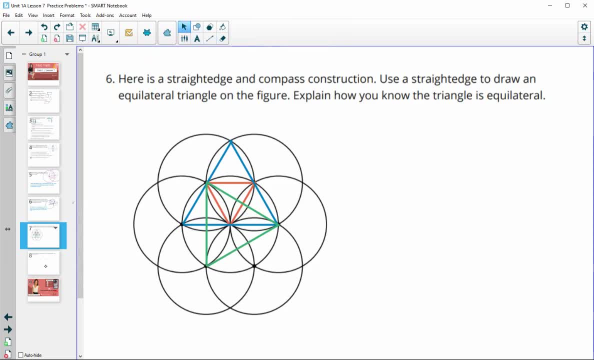 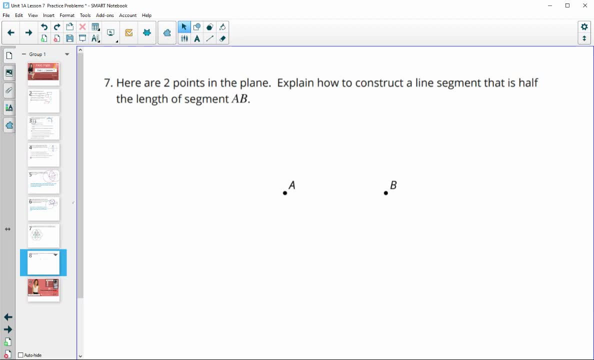 these pieces, computers can have the same measure of room, so any of those are fine. there's multiple others you could come up with as well. number seven: so here are two points in a plane explain how you could construct a line segment that is half of the length of segment a B. so let's go. 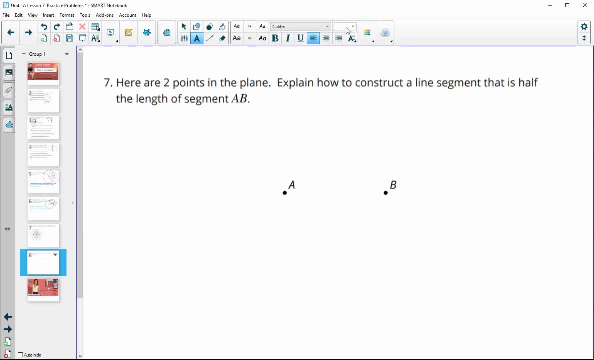 ahead here and start typing this out. so first of all I would say: connect points. connect points a and B to create segment a, B, and so let's just kind of do this. I'll do this as we type it. so connect. and then now the idea would be: 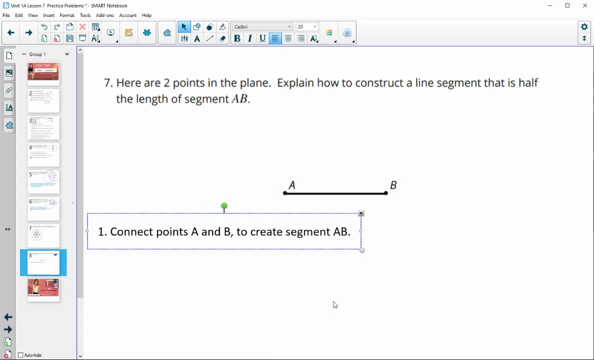 that we're going to do a perpendicular bisector construction here, because then we'll be able to figure out where the middle is. so, second, we would construct two circles centered at a and B, both with a radius of a- B. so you could, you would use your compass here, I'm just 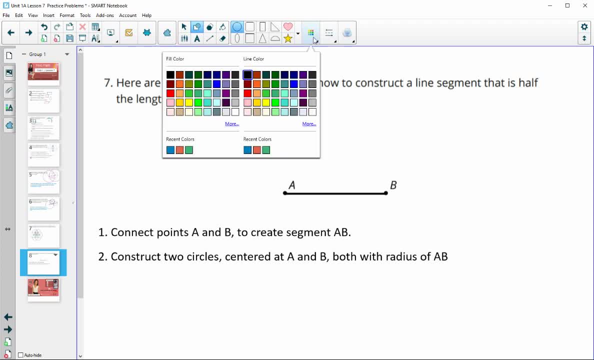 going to use the circle drawing tool, so we would let me make this a different color here and a little bit smaller. but so you draw a circle around a that has a radius of a- B. you draw a circle around B that has a radius of a- B as well. to